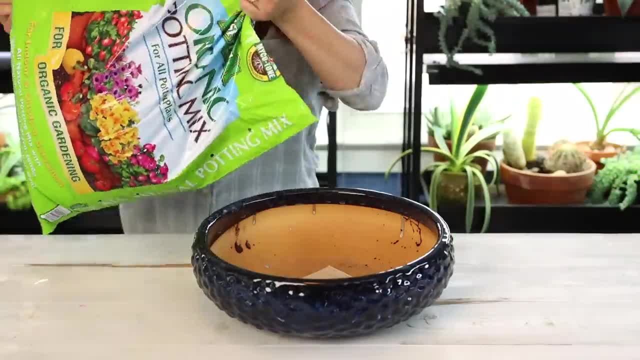 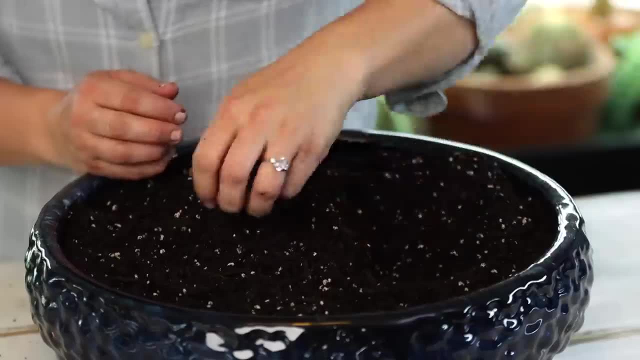 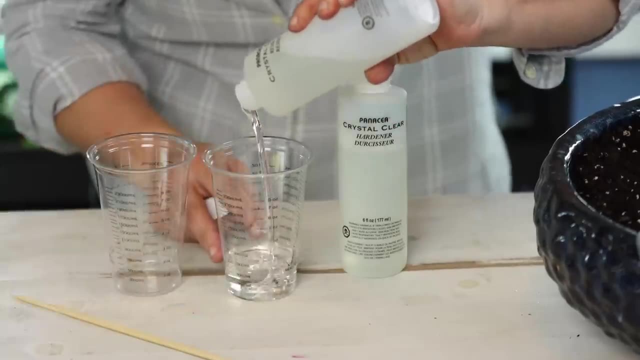 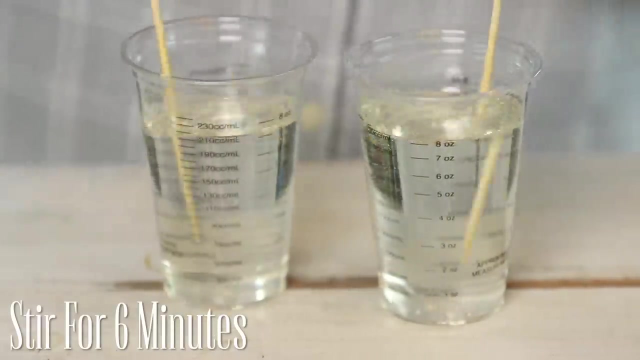 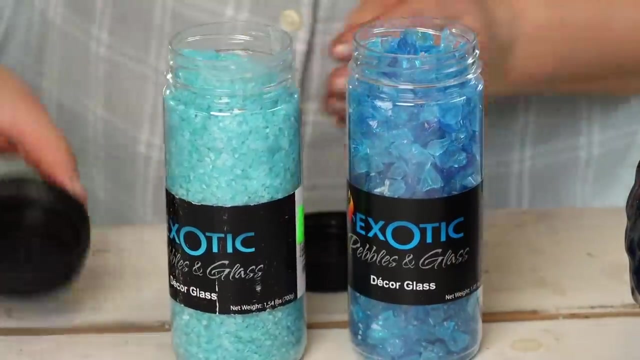 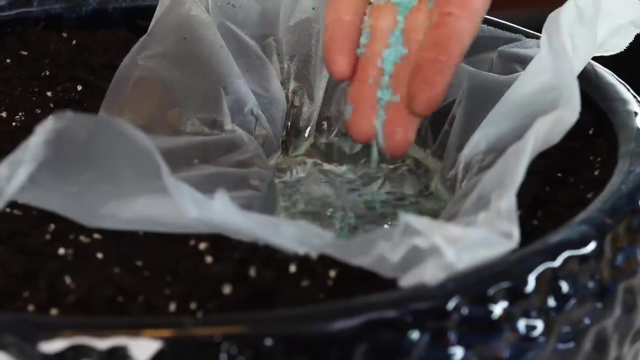 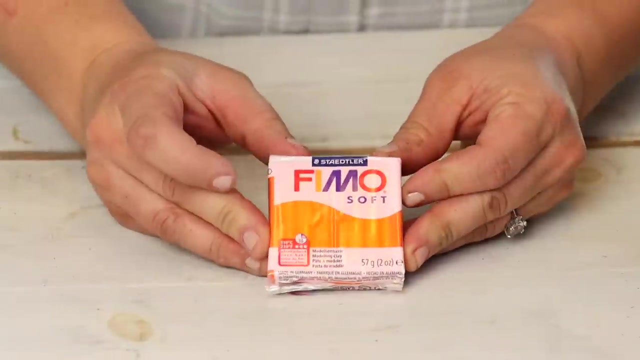 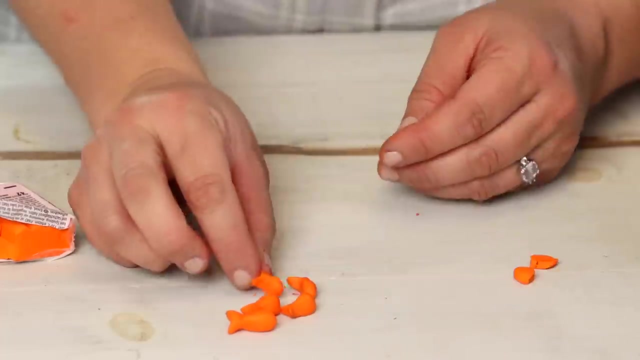 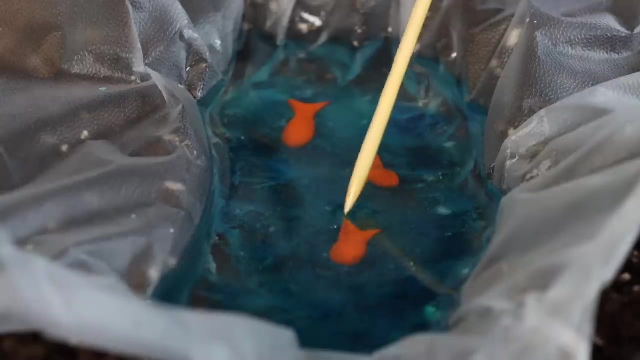 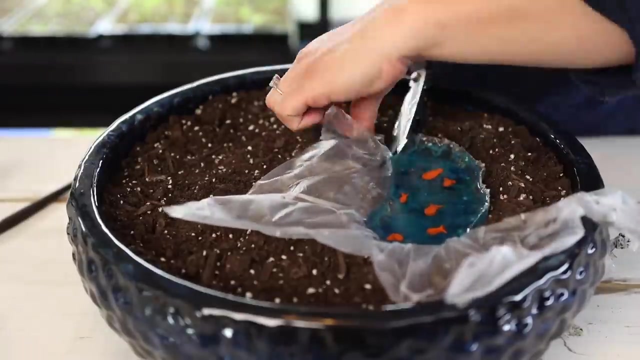 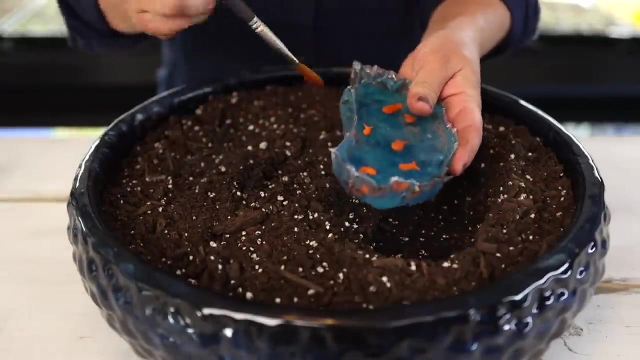 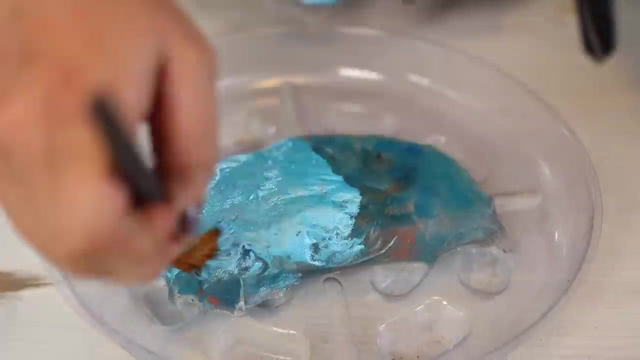 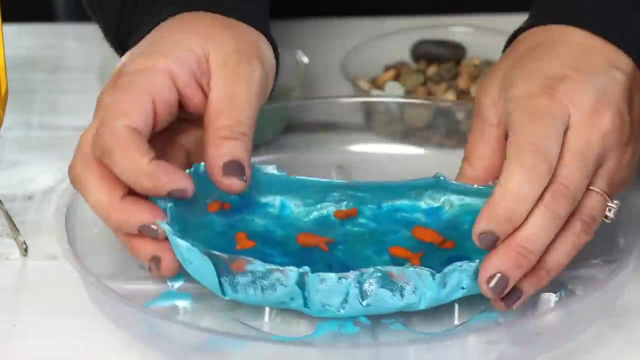 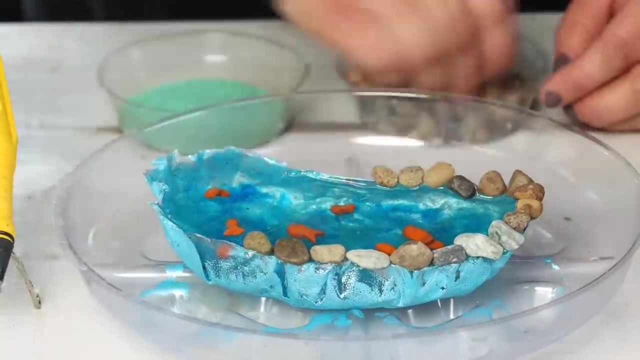 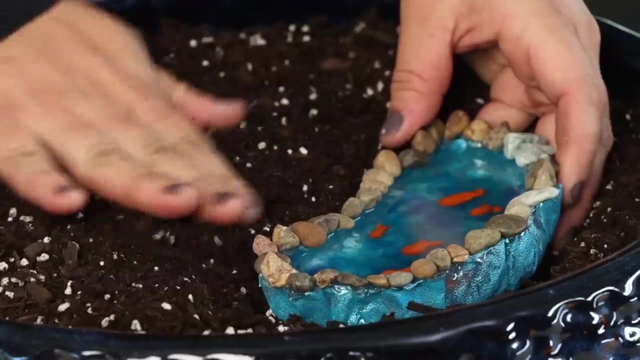 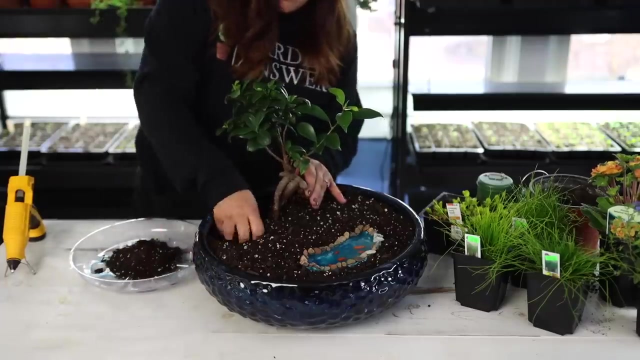 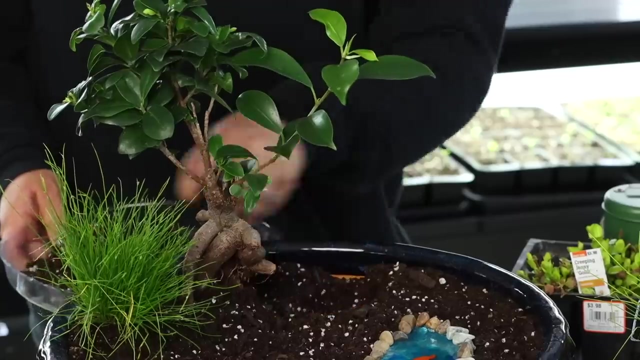 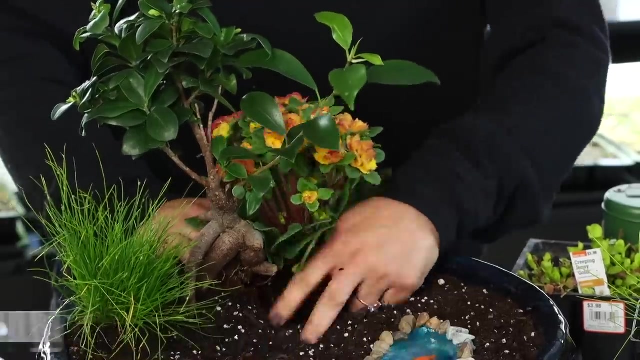 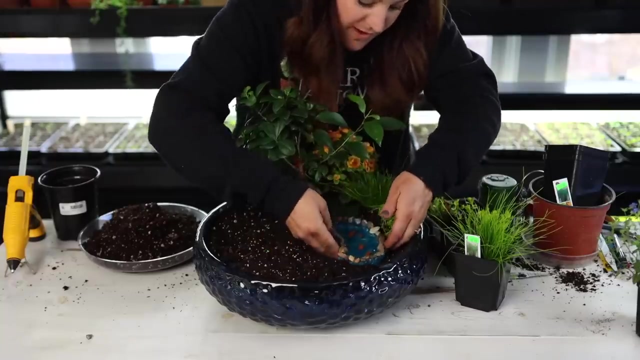 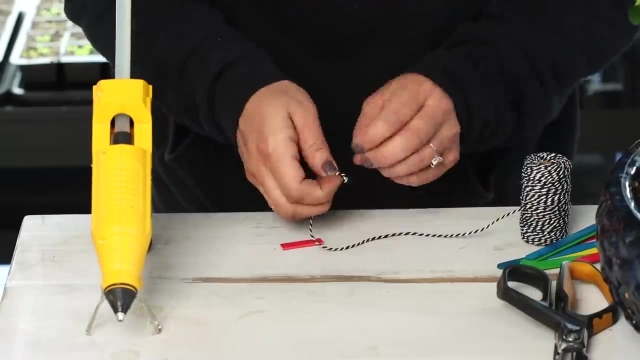 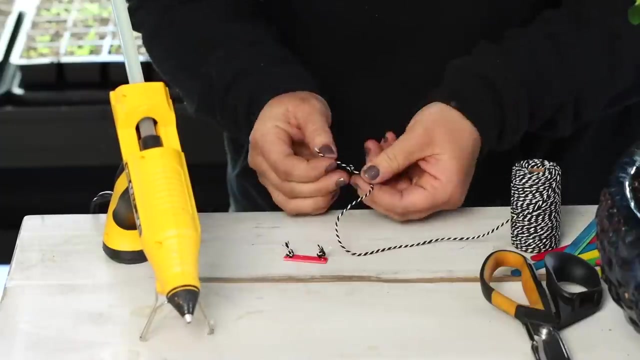 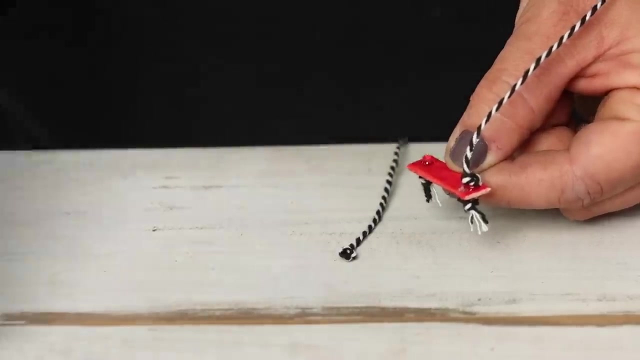 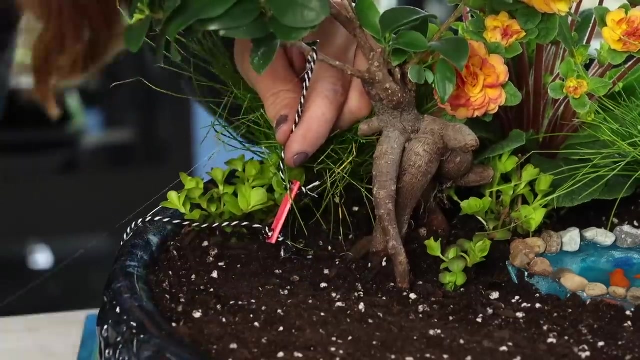 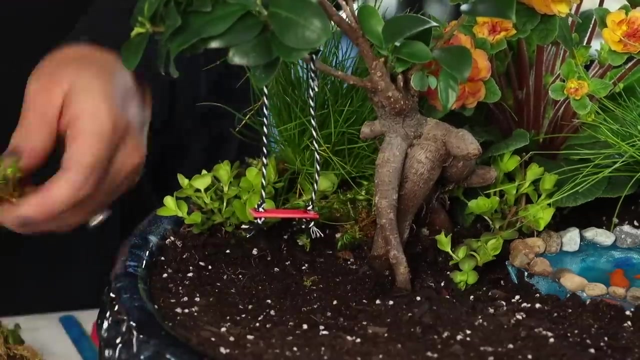 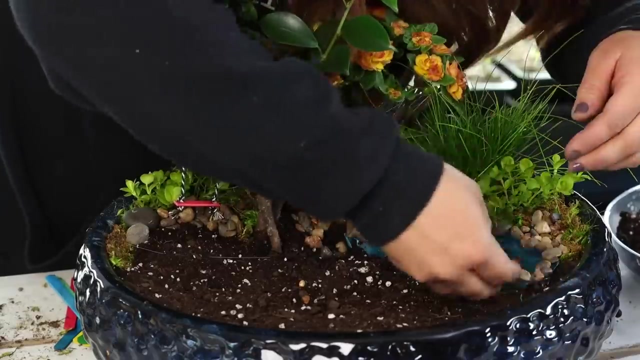 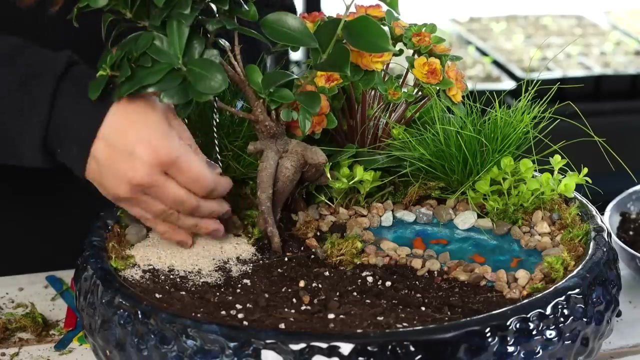 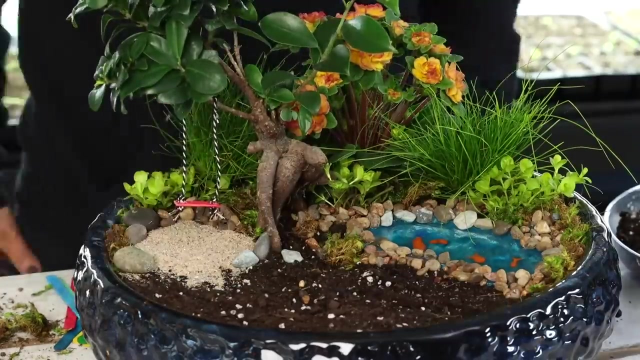 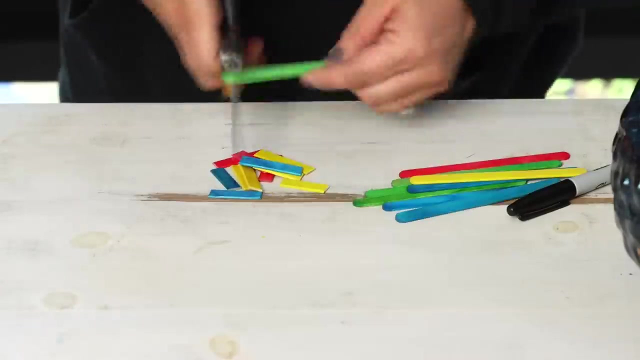 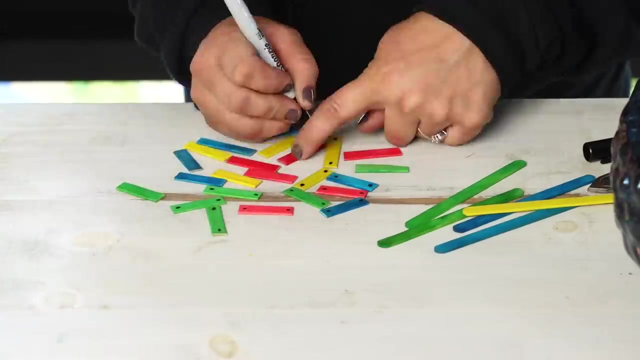 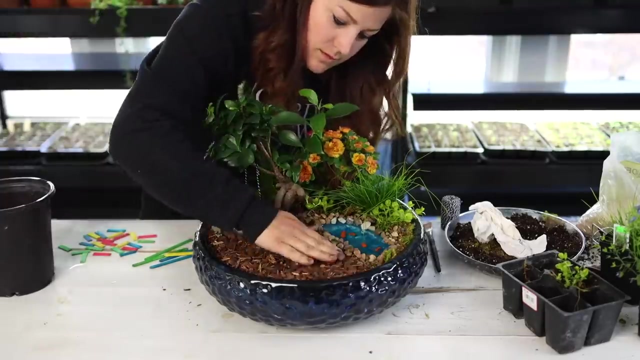 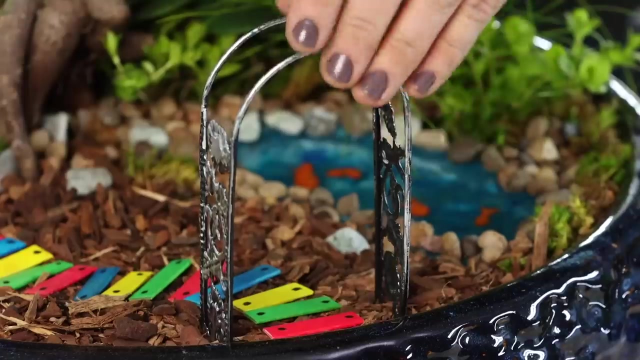 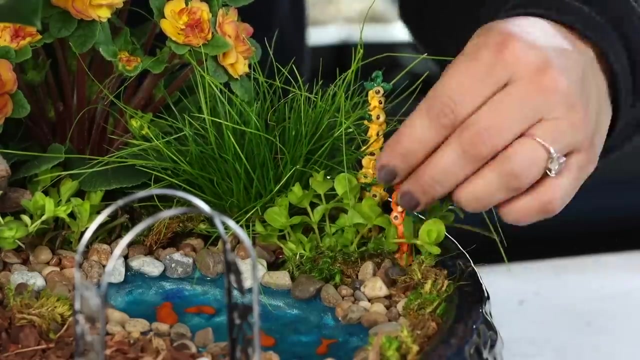 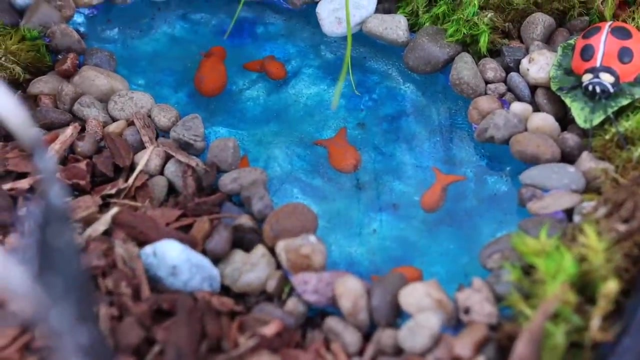 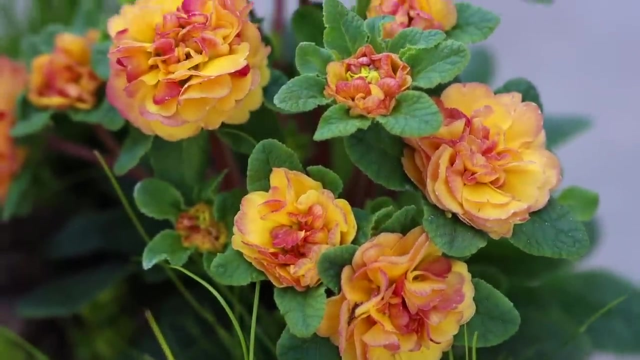 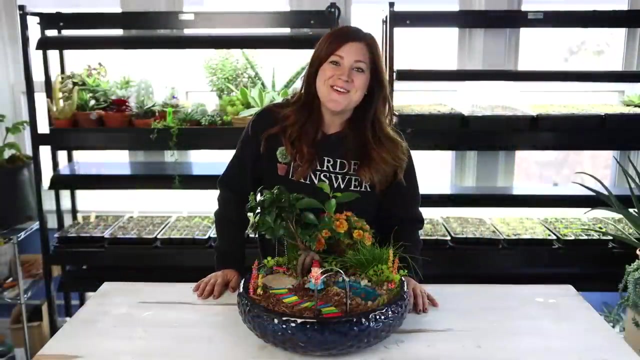 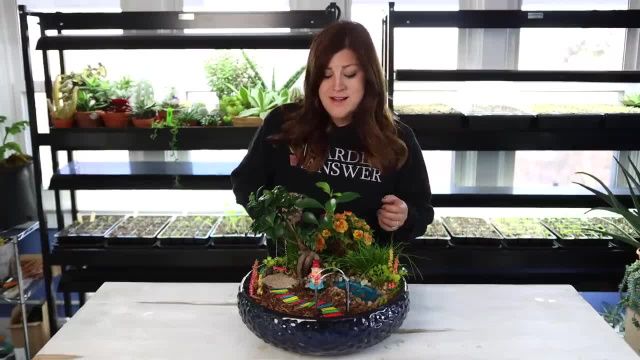 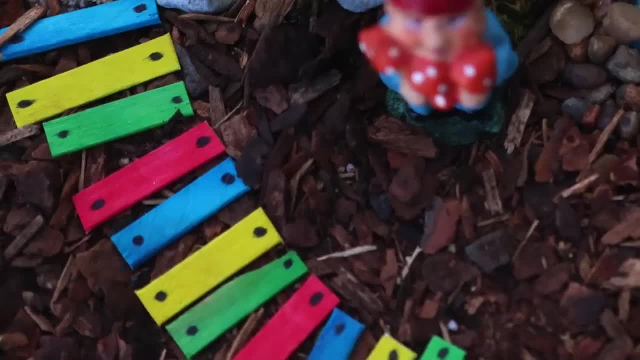 really kind of childlike and colorful and whimsical, and it incorporates a few elements that I think are really fun, like the colorful pallet walkway, popsicle stick walkway and this little pond that I had never tried making this before, but I had some leftover floral. 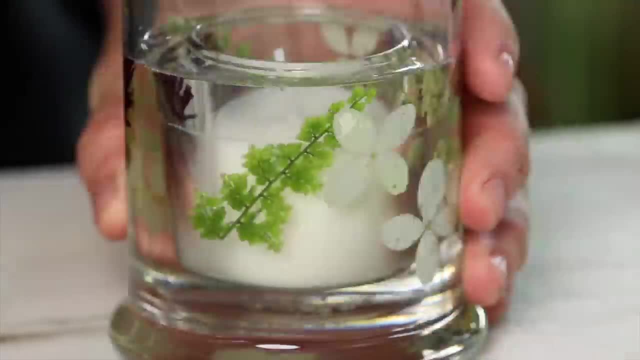 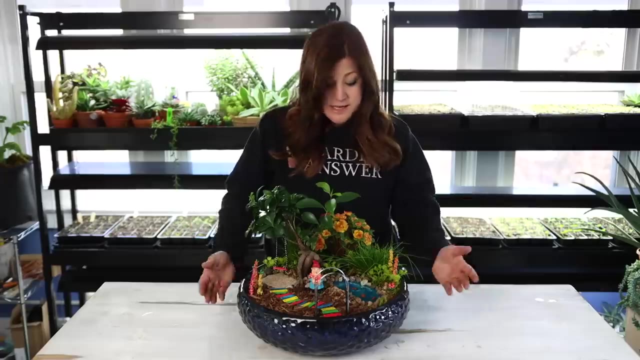 setting resin from our dried flower candle project from not that long ago. but I made so many candles that I decided to try using it in some other way. So what I did it was I got my container, got this down at the garden center. this is one my 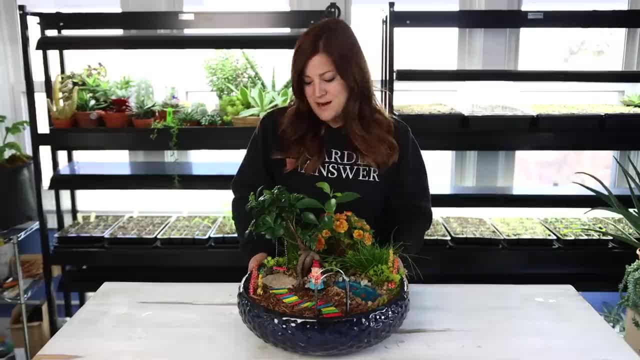 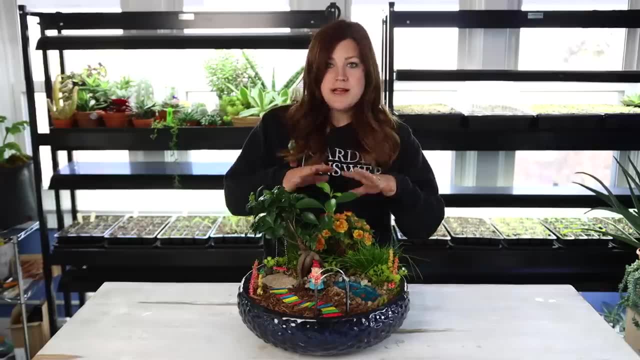 mom was displaying the day. I went and helped with spring setup and I just really liked the shape of it and the color of it and the texture on the side and I thought it would make for a really good either miniature garden or like a low arrangement for the middle of a table. I filled it with soil. 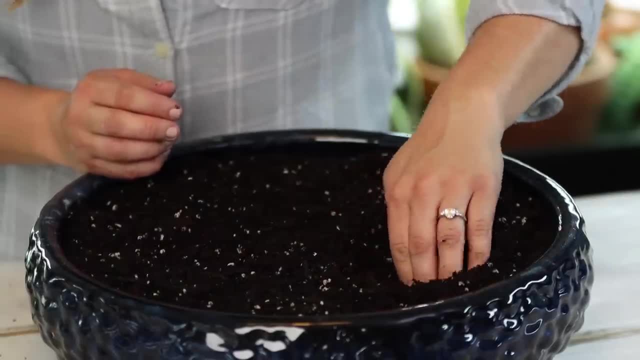 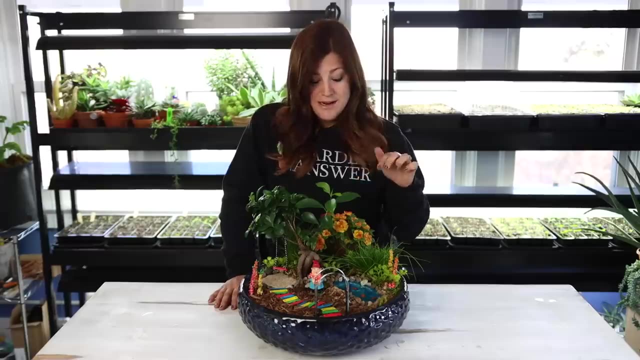 and then made a little reservoir or a little well in the soil kind of in the shape I wanted my pond to end up in, and then I lined it with plastic wrap, which I'm thankful I went with plastic wrap and not something different, because the resin ended up sticking to it, so it's clear enough that I was 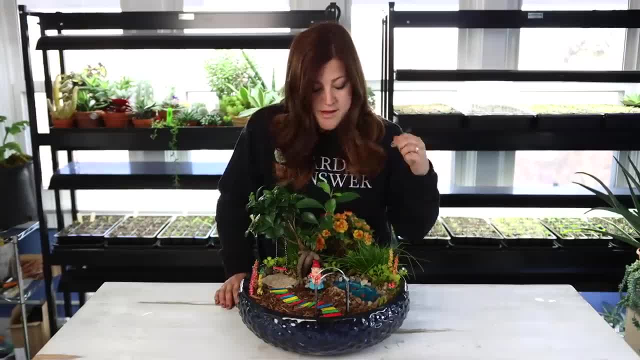 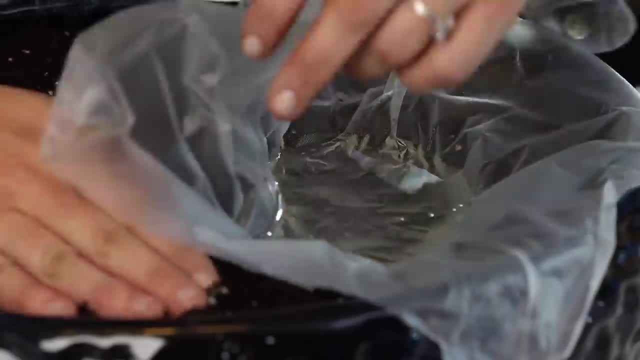 able to paint the bottom of the pond and I still got that really nice blue vibe. So I mixed up the resin, poured it into the pond and then I kind of like built soil around, like I kind of lifted up the plastic wrap and built soil up to where I ended up with the exact shape that I wanted. 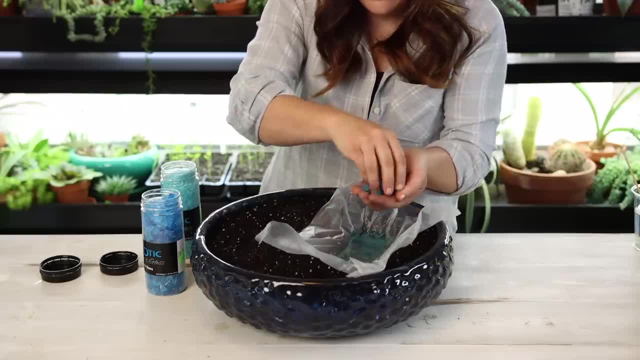 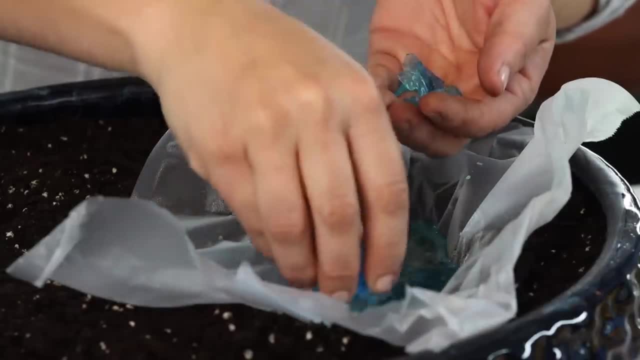 and then I sunk some stones down in the resin So I had some really fun like crystally looking, dark blue, like a teal, aqua color and clear, and they just sunk right down in there and it gave it a really neat kind of like mottled look and some. 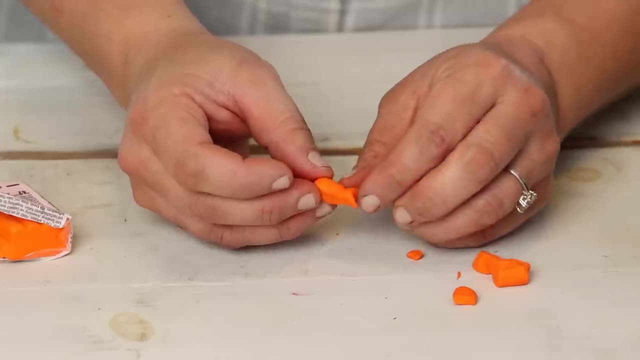 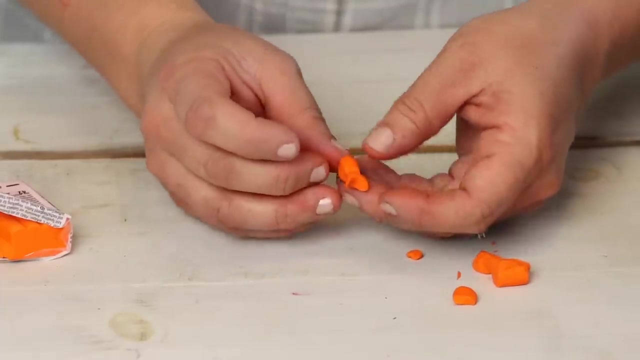 variation of color. I made the goldfish out of air dry clay and that was fun. I didn't know how it would turn out because I didn't let them dry all the way. I only let them dry for a couple hours just sitting out. I didn't bake them or anything, and they didn't color, bleed into the resin, which. 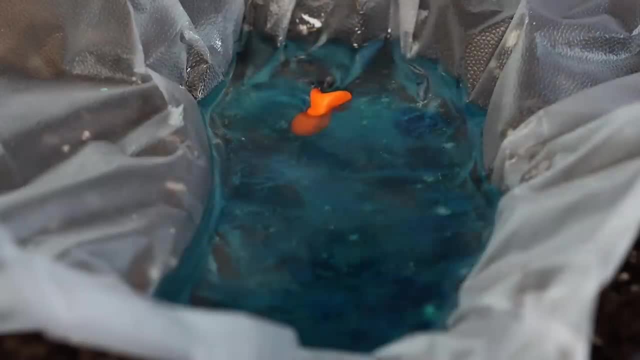 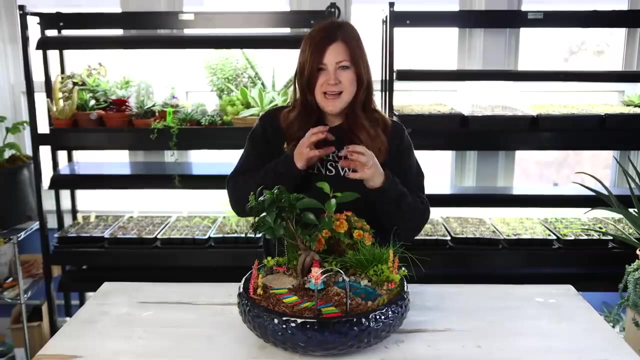 I was worried they were going to do that and I ended up. so it takes the resin like 12 hours to set. So I popped the goldfish in and then I came in later and kind of popped them into like, poked them into place once it had gelled up just a little bit more, and then it did take several. 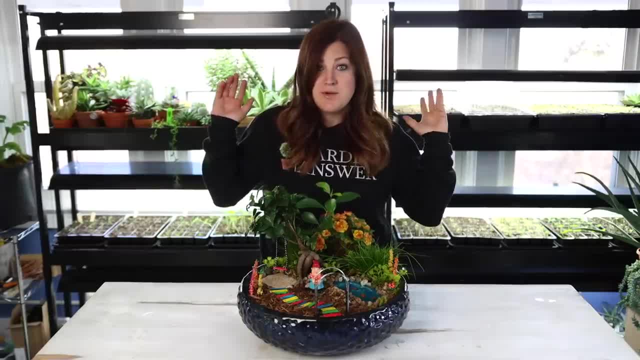 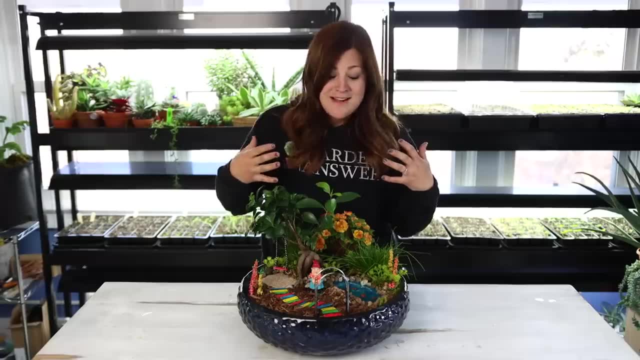 days for it to actually set completely hard, because we're in the plant room right here and this is where it was sitting. There's a lot of humidity in the air in this room, and so it was having a hard time drying out. Had I moved it to a different spot that's drier, it would have. 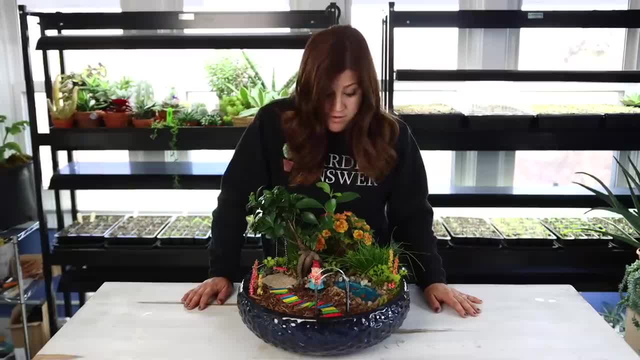 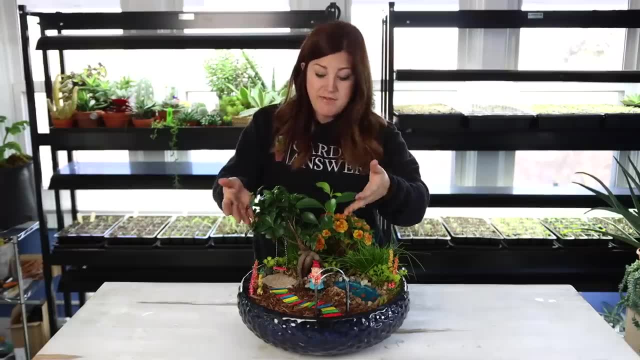 set up within 24 hours. So after that I'm trying to think of where I even started today. I think I planted my tree first. This is a ficus. They just got these down in at the garden center and I thought it would be the perfect choice for. 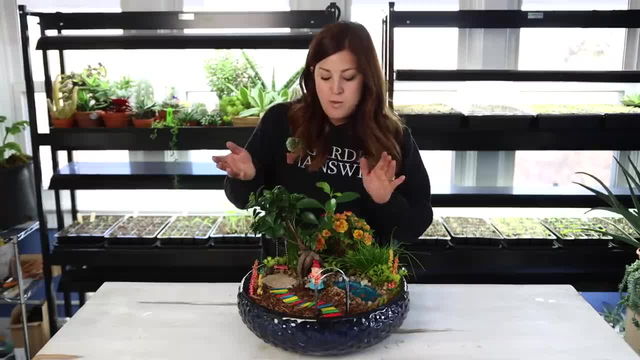 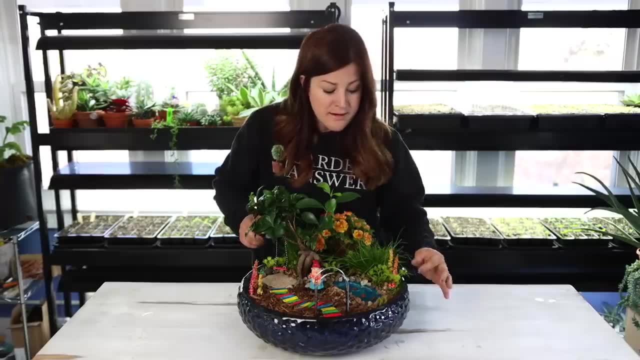 this arrangement because I really wanted to make a little swing and hang it off what looks like, you know, a big tree. in this arrangement I have a couple of fiber optic grass, which is kind of perfect for around the pond. I had some creeping jenny- goldilocks creeping jenny- that I wintered. 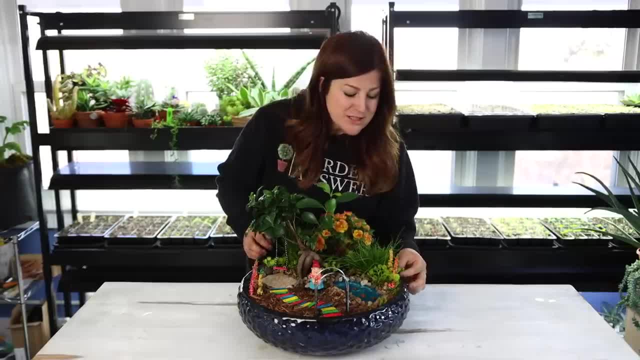 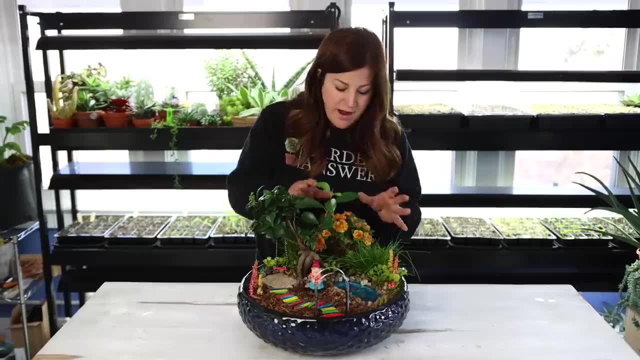 over in our greenhouse and they were. I cut them all back, so they're just starting right now and they look really fresh and like perfect size. and then a bellarina nectarine primrose, which this one- the flowers will eventually fade. There are a ton of beautiful flowers that I'm going to. 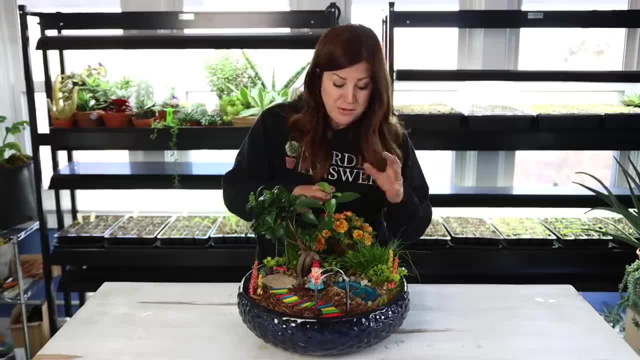 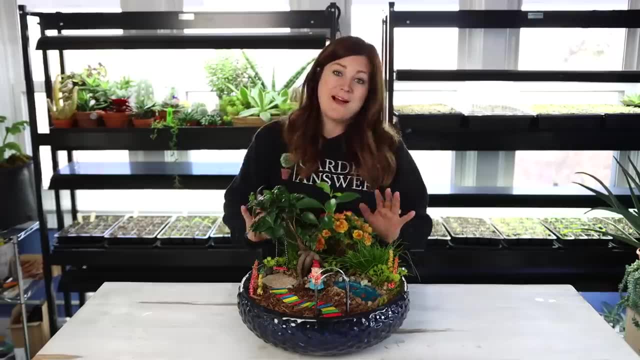 show you in a little bit. I'm going to show you a bunch of little buds down in here, though, Like they are just coming up like crazy, so I think we're going to have a really nice long show. So I didn't use an enormous amount of plants and I backed them all up toward the back just to create. 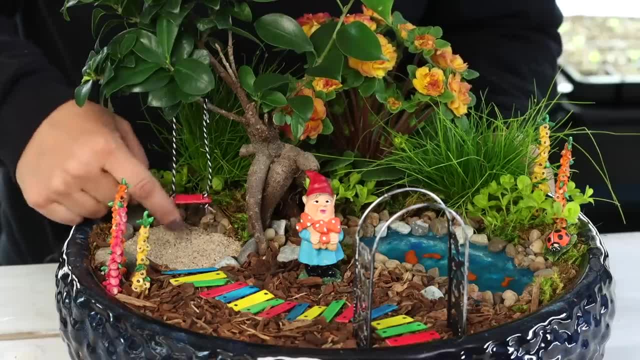 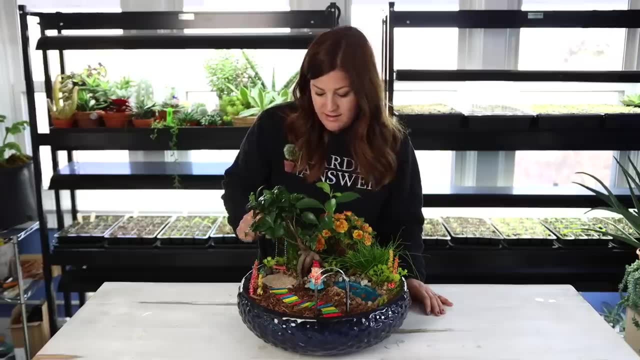 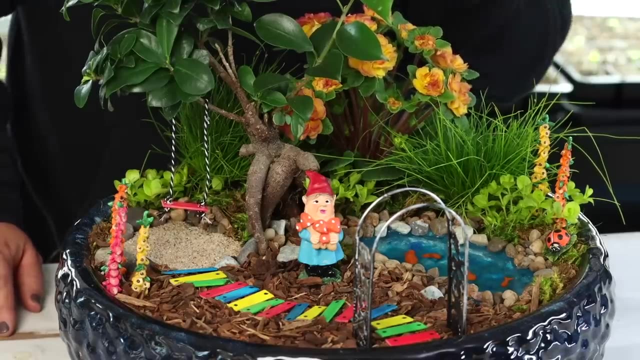 a nice backdrop for everything going on in front, A little sand kind of like you see in a playground. you either see like gravel or sand, usually underneath where the swings are, and so I thought that that was kind of perfect. And then I found a bag of colorful popsicle sticks. I didn't like. 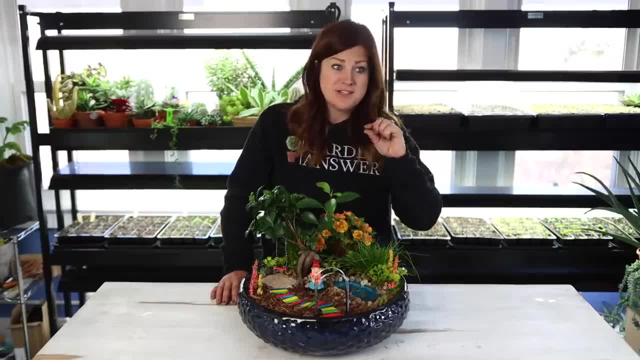 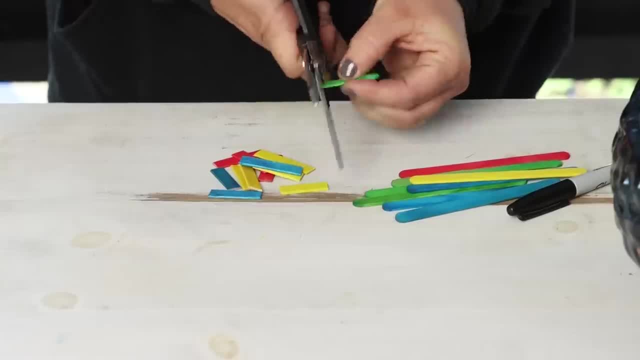 they've probably been around forever. I didn't even know that they existed. So I'm going to show you what I did. I was just going to go look for regular, just wood colored popsicle sticks, but I saw these and I thought, oh, that will be just so perfect for this garden And I just used a pair of scissors. 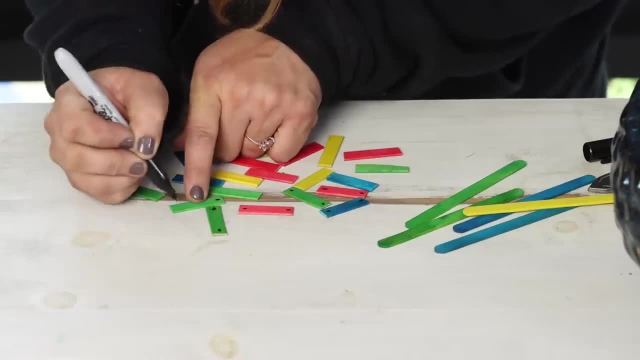 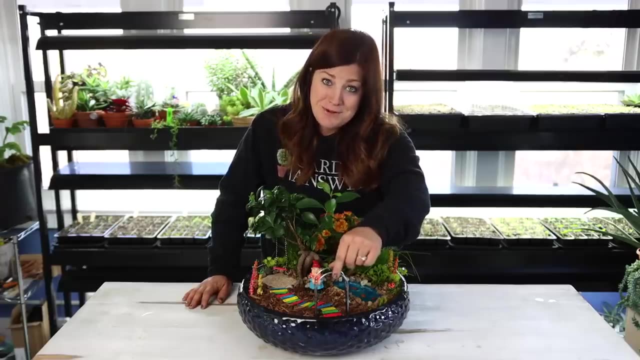 to cut them, and then I put a little black dot on either side, kind of was like our landscape pins, like I used on our pallet walkway behind our chicken coop. These two pieces right here were actually sent to me by one of you guys. So, Abby and Nicole, thank you for the package of miniature. 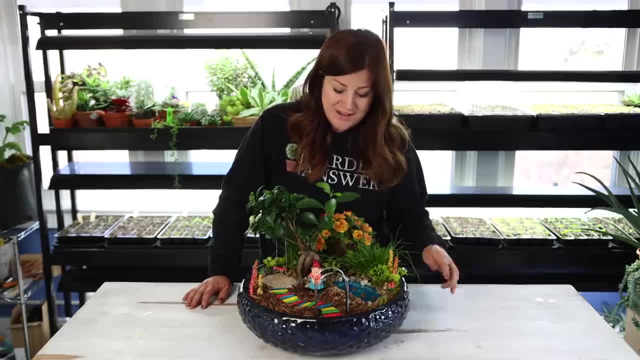 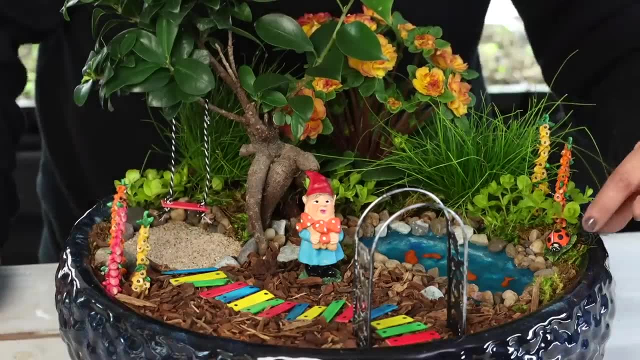 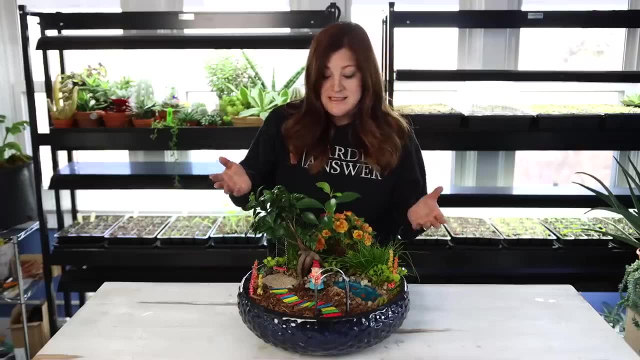 pieces you sent over. The other ones I'll probably work into other miniature gardens, but I thought these fit in perfectly with this particular garden. And then I had some hollyhock, this little picks, and this cute little ladybug that I incorporated in, and I just think it turned out like just so sweet. So this arrangement, right here it's.